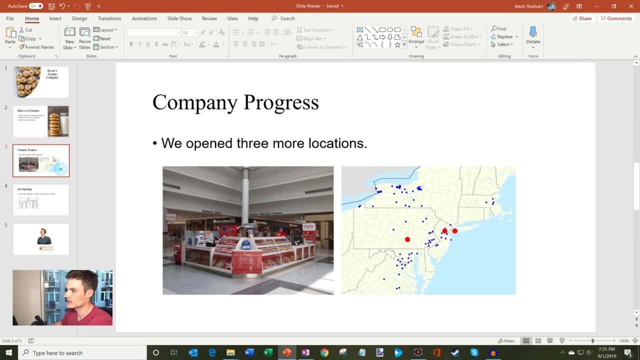 of cookies and the full glass of milk. because we're optimists And company progress. we opened three more locations and I show all these other locations because we're already a very successful company. You wouldn't want to miss out on this investment. And then we 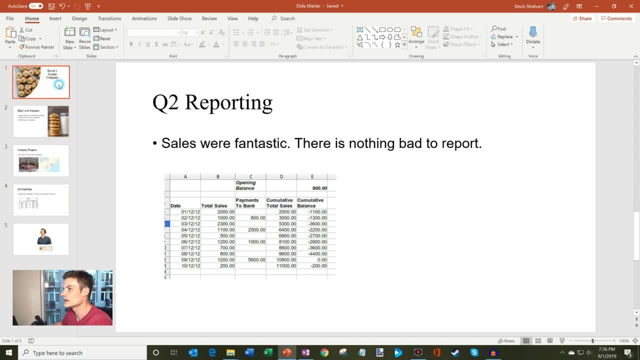 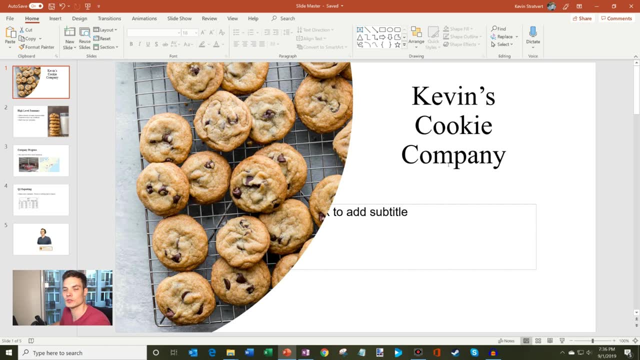 also have our Q2 reporting and sales so far are looking great. Okay, so a few things with this deck that I want to update. Times New Roman: Who uses Times New Roman anymore? It's a font I used back in high school. 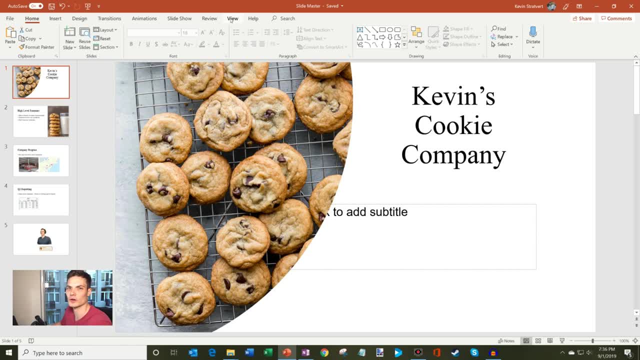 That is just a dated font. Let's update to something more kind of more contemporary. The way we do that is click on View and within View you have something called Slide Master, And let's take a quick look at this description here. So master slides control the look of 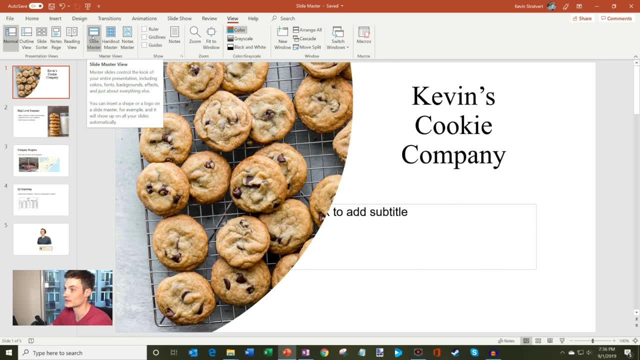 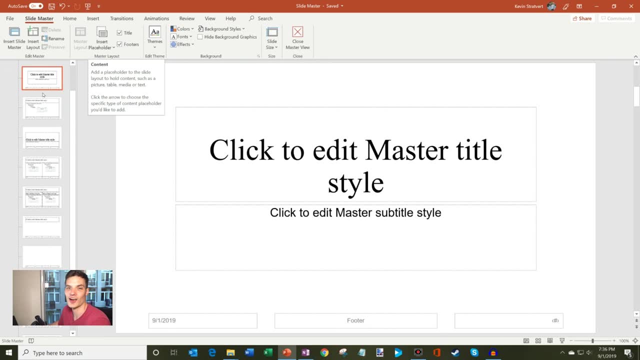 your entire presentation, including colors, fonts, backgrounds, effects and just about everything else. You can insert a shape or a logo on a slide master, for example, and it will show up on all your slides automatically. All right, Well, I won't believe it until I see it. So what we're going to do now is, I mentioned, 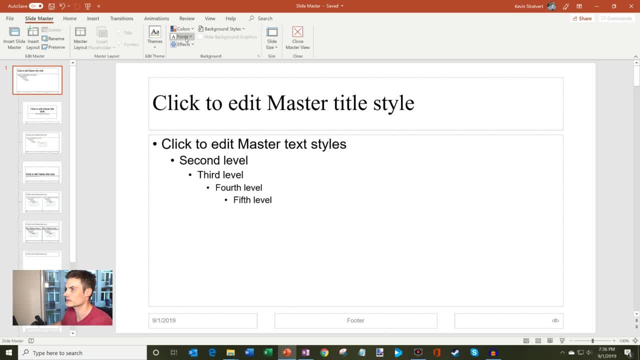 we have this Times New Roman font and we want to modernize that. So I'm going to click on Fonts up here and what we could do is we could select Segoe. That's a nice, more modern font, So let me select that. Some other things you could do is you could edit colors. you. 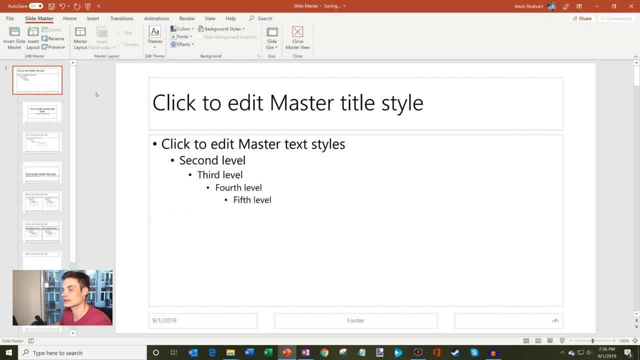 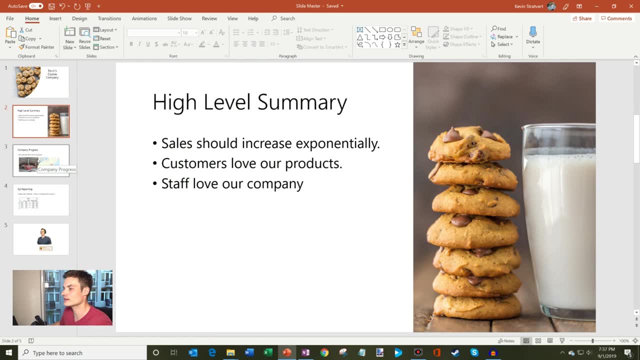 could set effects, you could set themes for all your slides, And let's take a look and see what happens. So I'm going to click on Close Master View And so now what you'll see is the font has updated on every single slide in my PowerPoint. 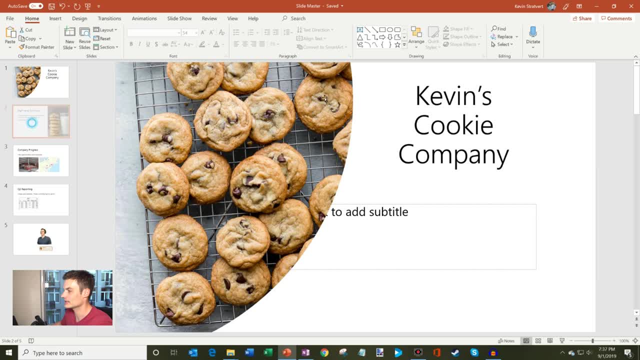 presentation. Now, instead of having to go through slide by slide by slide and update all the fonts there, I've just updated it in one click, basically through the slide master. Some of the other things I might want to do, let's say, maybe showing the logo of my company. 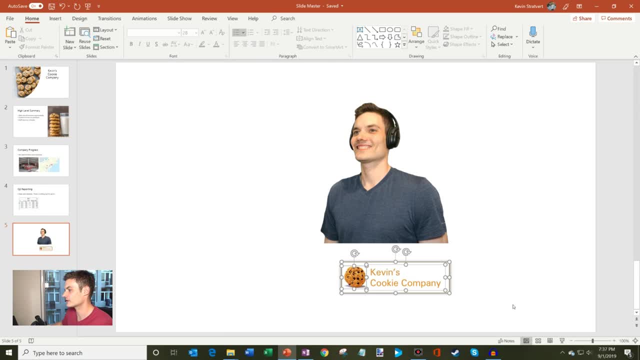 on each slide would be a nice touch. So I have this beautifully designed and crafted logo. Actually, no, that's kind of dreadful, but I just needed a quick example to show how you do this. So here's my Kevin Cookie Company logo. I'm going to copy that and I'm going to go back to the slide master. Let's see, So I'm going to go back to the slide master. So I'm going to go back to the slide master. Let's see, So I'm going to go back to. 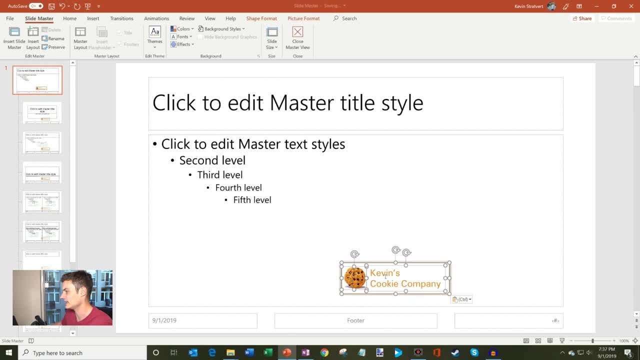 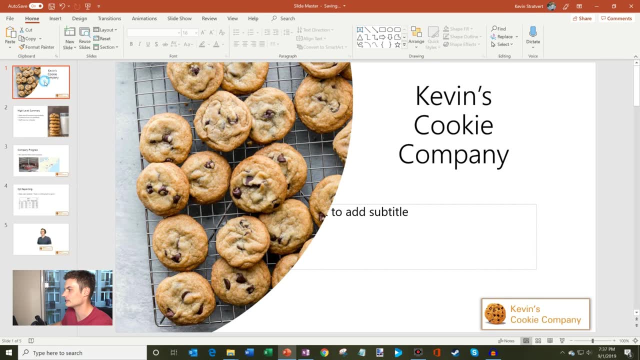 the slide master. Let's go back to the slide master and I'm going to paste it in, let's say, the bottom right-hand corner, so it shows up on every slide. And now I'm going to exit the master view again, and there you see, my logo shows up there and here and here. Why? 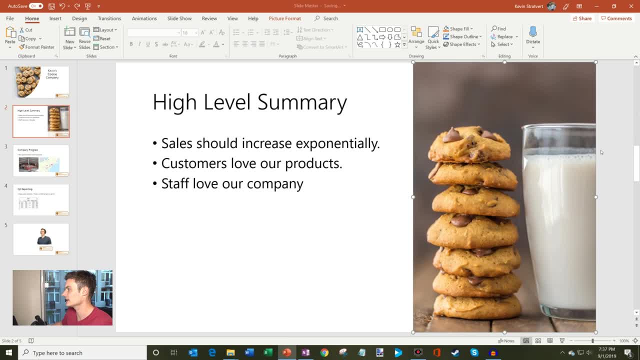 doesn't it show up on this slide? Oh, my image is hiding it, But you get the idea. It'll show up on every slide as the lowest layer on those slides. By the way, if you're looking at learning about layers, I have a tutorial video on that that you could check out in. 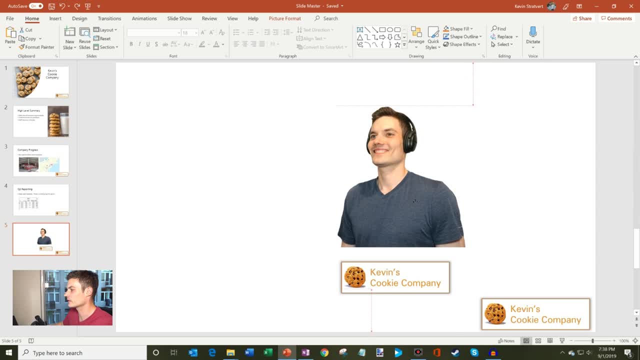 the description down below. And let's say that I want to engage the slide master. So I'm going to go back to the slide master and I want to include a photo of the owner of this company. So maybe I reduce the size and I want to place it right above the logo. So let's go back into the slide. 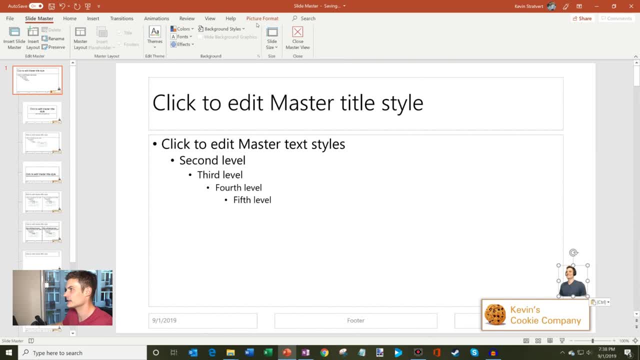 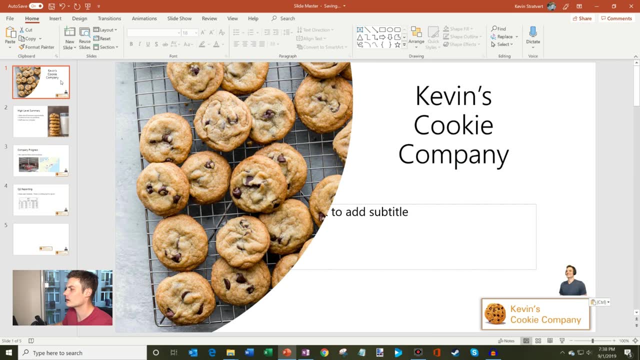 master once again, and we could paste it in, and there it shows up above my logo, on every single slide. And let's say that I only want it to show up on the title slide, but no other slide. Is it possible to do that, or does it just apply to everything? Well, no, you could. 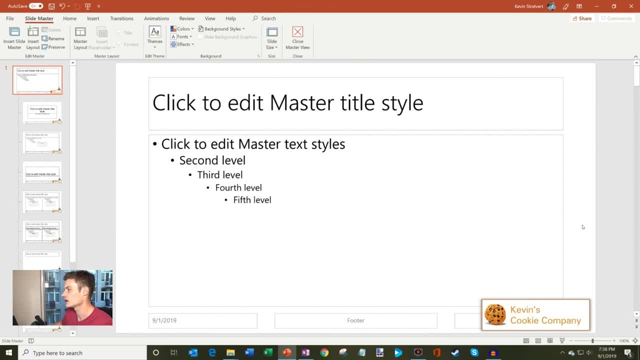 just do it to an individual slide. So what I'm going to do is I'm going to remove my logo, remove my title slide and sort it out from this master slide. that applies to everything, And what you can see is these are all the different layouts you could select when you 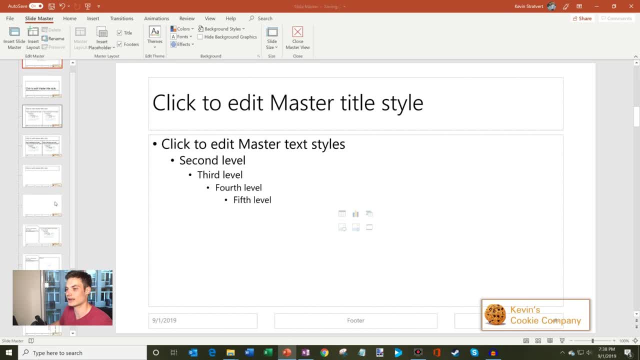 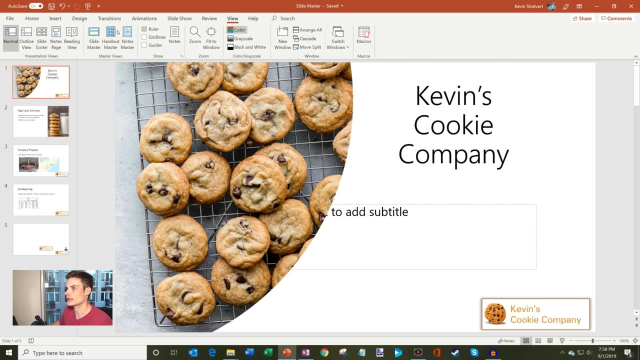 create a presentation. You have your title layout, you have your content layout and so on and so forth. If I go back here, this maps to all the different layouts you could choose when you insert a new slide. Okay, so let's jump back into the master. And I said I only 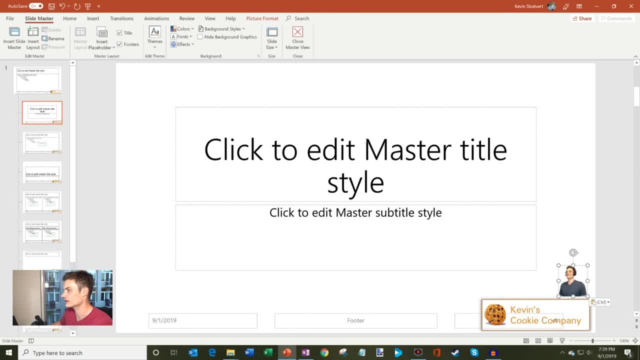 want to add it to the title slide. So I'm going to go to the title slide here and then we're going to paste in my little picture. maybe it's kind of peaking up from the logo And let's bring. yeah, that looks good. 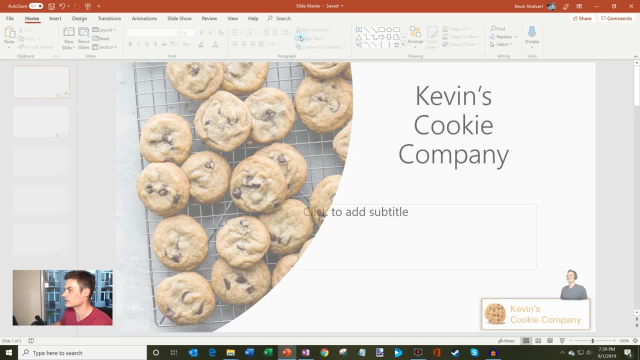 And so what you'll see is it shouldn't be on any of the other slides. And now we're going to close the master view, And so here I show up on the title, but I don't show up on any of the other slides. 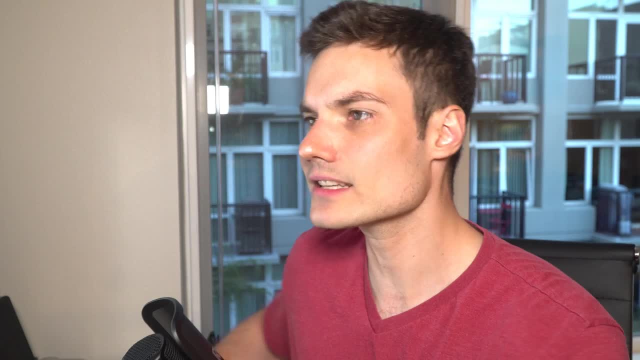 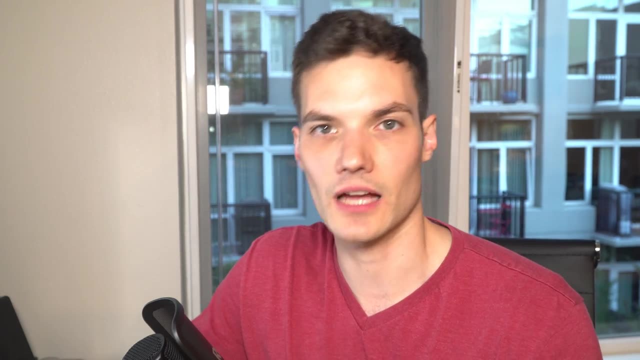 But it doesn't show up on any of the other slides. So that's a quick, just a quick- tutorial of how you could use master slides to update things through a very large deck very easily, whether it's colors, fonts, imagery, any type. 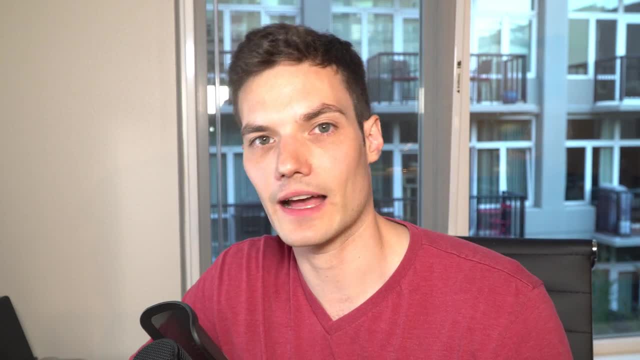 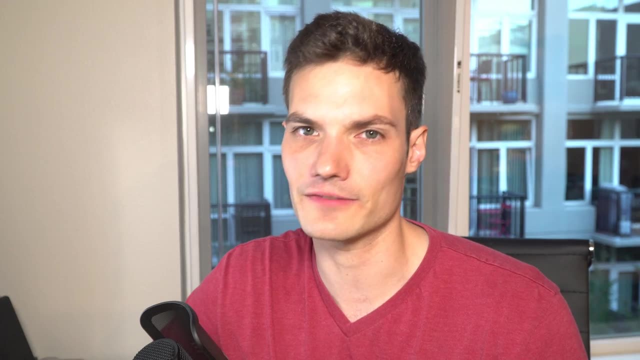 of content on the slide that shows up in a number of places. It really simplifies the job of updating or adding to many slides. So hopefully, if you were able to use the slide master and it helped save time when you were creating a presentation, please hit that like button. 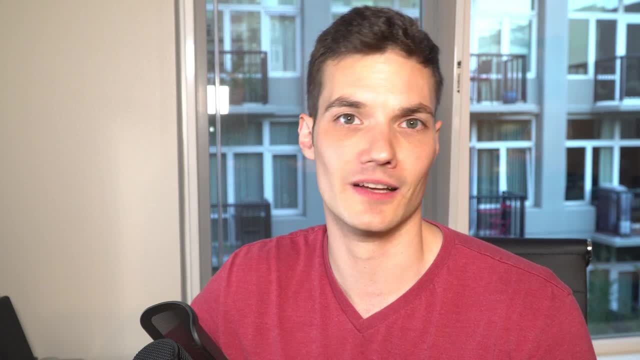 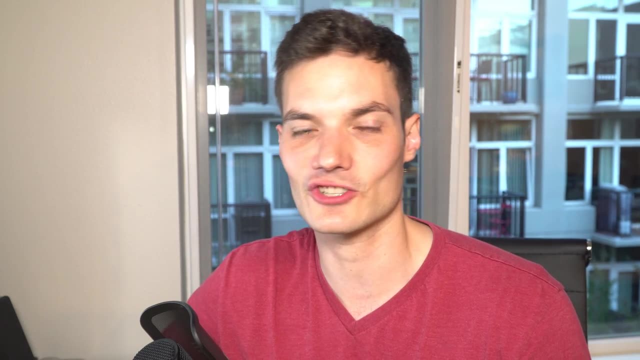 If you want to see more videos like this in the future, more tips and tricks for Word, Excel, PowerPoint or any other things that I decided to create a video on, feel free to hit that subscribe button. That way you'll get a notification.